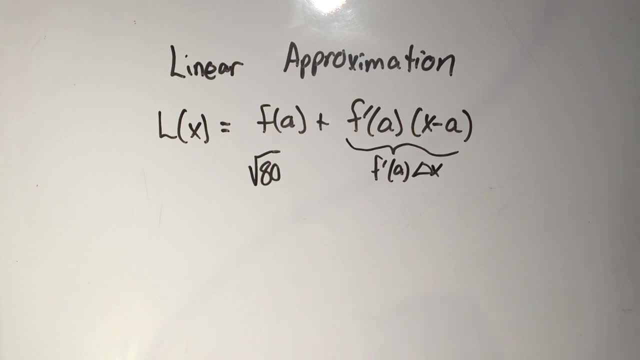 times x minus a Delta x or like the change in x, But this is how I prefer to write it. So if you had a function and an a, you could write the linear approximation for anything. So what is the function I'm concerned with in the square root of 80?? Well, I'm concerned about the 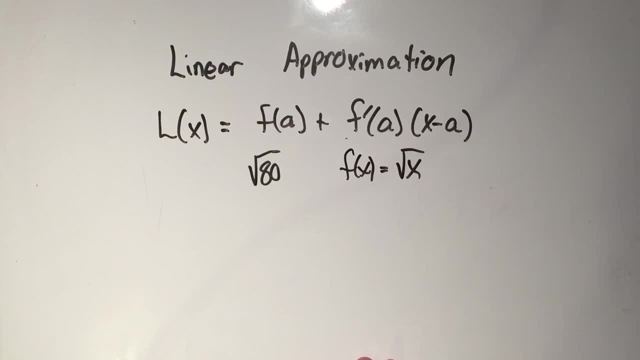 square root of 80.. Well, it's the square root function, And a is a point close to 80 that's easy to work with in the function. So what's something near 80 that's easy to take the square root of? How about 81?? Square root of 81 is 9, so that's really easy. So a is something near. 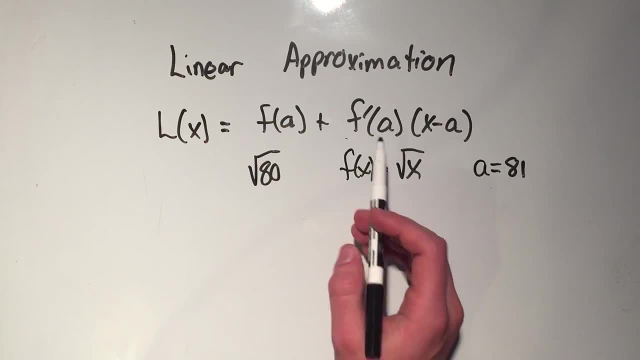 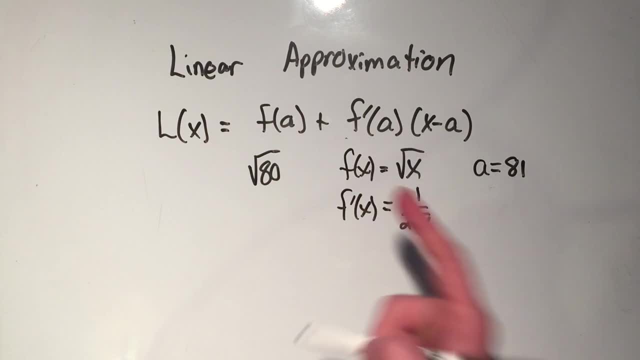 for derivatives of square roots. if you haven't seen that before, If you don't like that method, you can write the square root of x as x to the 1 half and then use the power rule: Bring down the 1 half x, subtract 1 from the power. 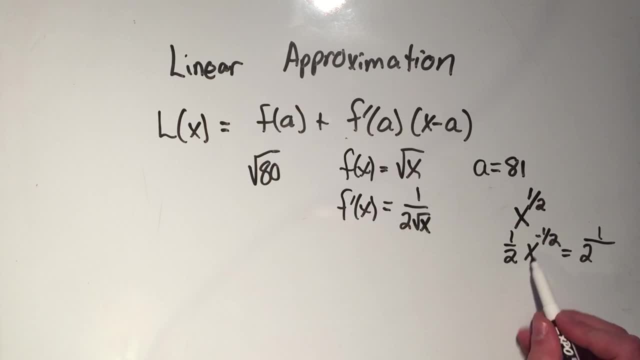 And then if you rewrite that that's 1 over 2.. Negative means on the bottom, 1 half means square root. So I just like to do: the derivative of a square root is 1 over 2 times the square root. 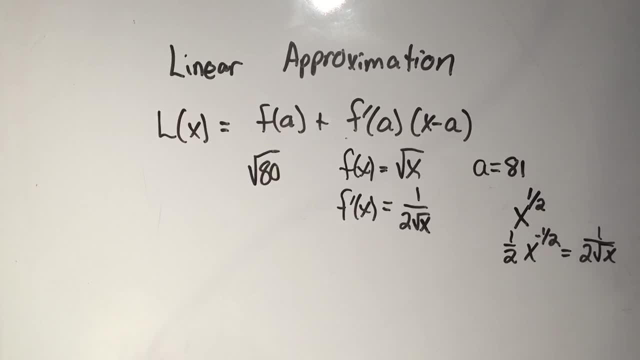 And if there's anything else in there, you got to multiply by the chain rule, But so I'd like doing that. There's a tip you weren't expecting on getting in this video. Okay, and now I can start filling this thing in. So my linearization, my linear approximation. 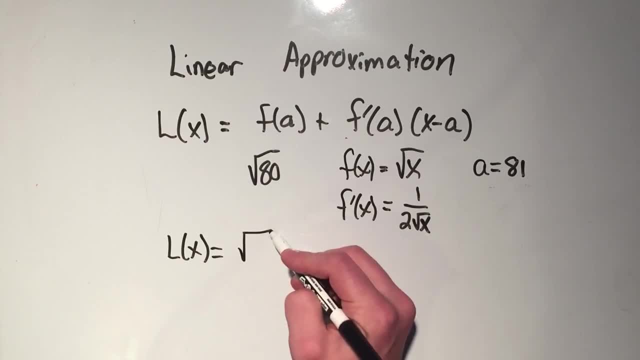 is f of a, That's square root of a, square root of 81, plus f prime, which is 1 over 2, square root of a. plug a into there. times x minus a. There's my linearization function And I can clean this up. 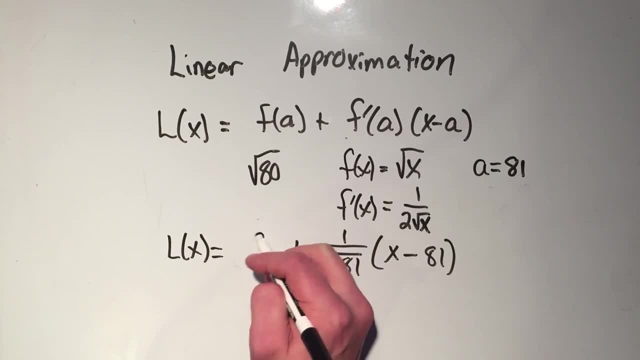 we know what the square root of 81 is, That's 9.. So this would be 1 over 2 times 9,, or 1 over 18.. All right now. so for values close to 81, this closely approximates it. 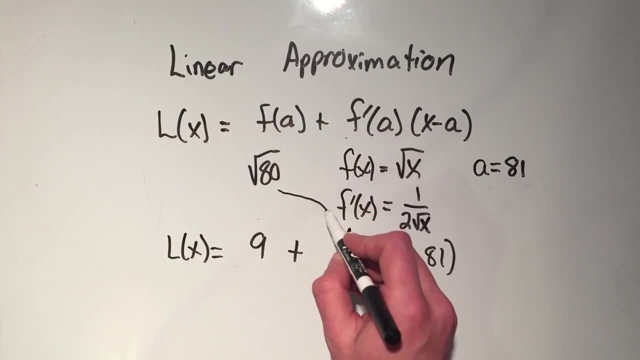 Let's plug in 80.. I'm going to plug in 80 right there And let's see what happens. My linearization of 80, that'll be 9 plus 1 over 18.. I shouldn't have drawn that arrow: 80 minus 81.. 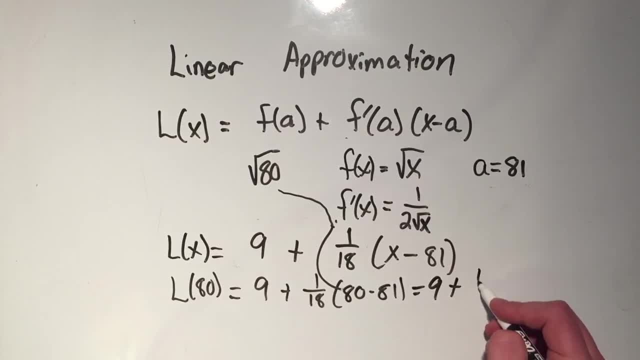 Well, that's 9 plus 1 over 18 times minus 1.. Or I might as well write that as just 19 minus 1 over 18.. And if you feel like it, you can get a common denominator. But I think I'm just going to leave. 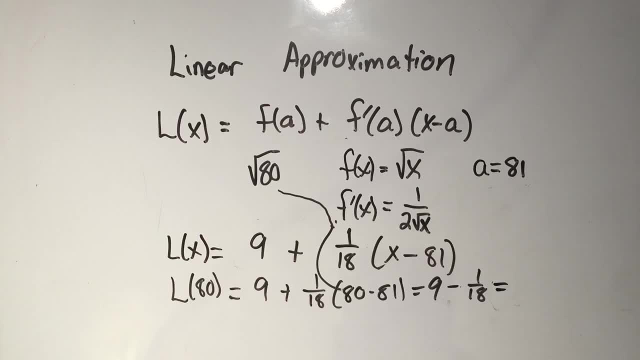 it like that. So now if I plug in 9 minus 1 divided by 18 into my calculator, that's 8.94 repeating All right, that's what our approximation is for the square root of 80.. Now if I plug into my calculator the square root of 80, I'm getting 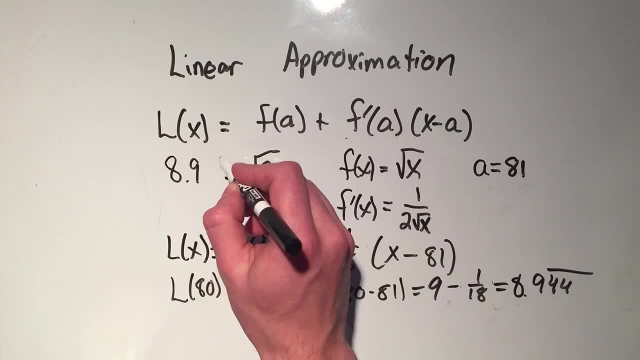 8.94427.. So, wow, that's a pretty good approximation. I'm within the limits of a place just by doing a little bit of derivative work. So if you did that for the island people, I guess they'd be pretty impressed And they'd say: OK, we'll let you live and use a. 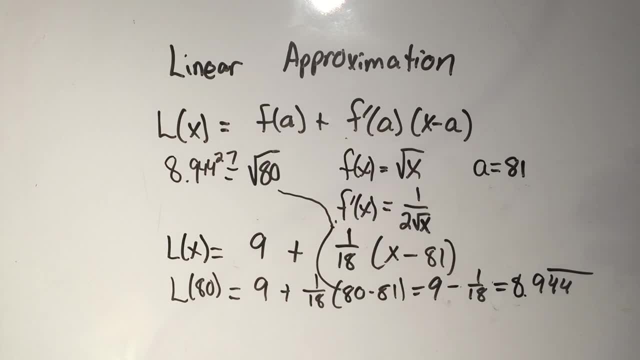 calculator again. Anyway, that's how you use the linear approximation formula. I just recommend you remember this And then from there it's just a matter of plug and chug on the test. OK, I hope you got something out of it. Please like and subscribe. Tell me what videos you want. me to make next And have a great day. Bye-bye.